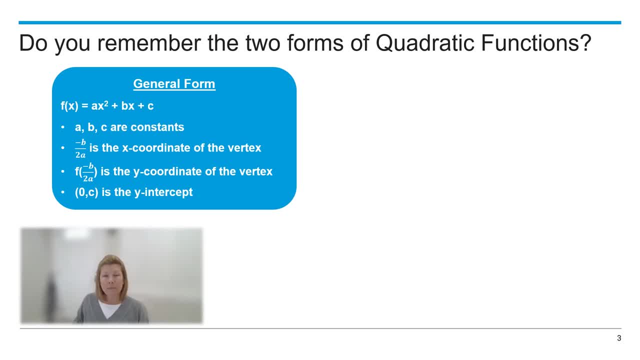 the y coordinate of the vertex And then, last but not least, the y-intercept. when you graph this equation, the y-intercept, or the point where this will cross the y-axis, is at the value z. Here you will find that the x-intercept is, And you also will find that in the equation. 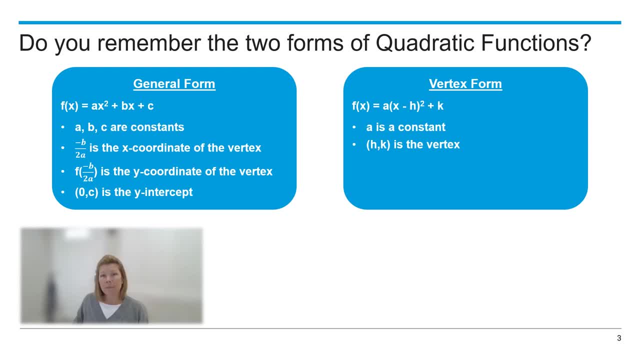 that comes in the formula. you have to plug that into the equation and then you are left with the original work of x squared and then you will find the y-intercept of the vertex. So you can see that the y coordinate is 1 minus 0, and the y coordinate is 1 minus 0c. 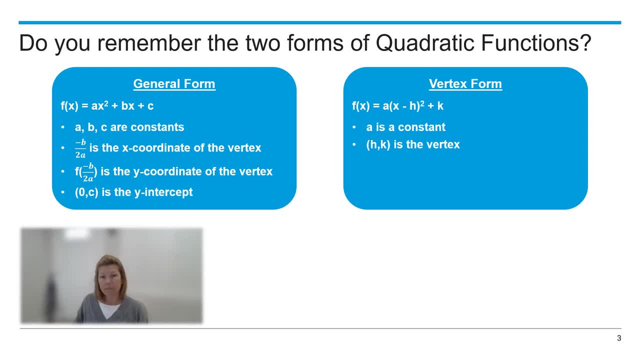 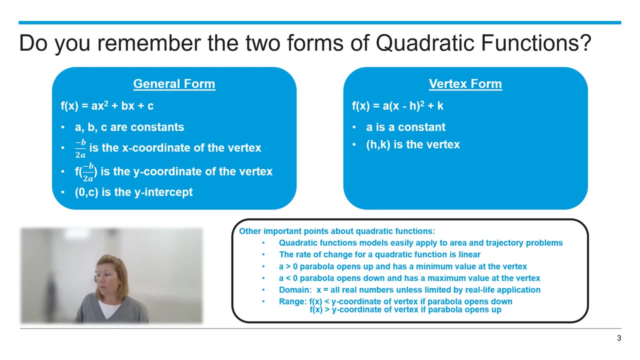 would be the coordinates of the vertex. Most of what we're going to concentrate on will be in the general form equations. Other important points that you should recall about quadratic functions include that their models easily apply to area and trajectory problems and the rate of change. 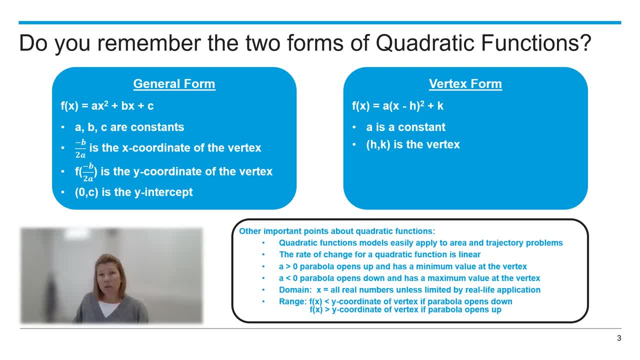 within a quadratic function is linear. I'm sure that might sound a little bit confusing, because a quadratic function itself is not linear, but the rate of change as you move from one point to the next is linear, and so we'll do a specific example to help you understand what we mean by. 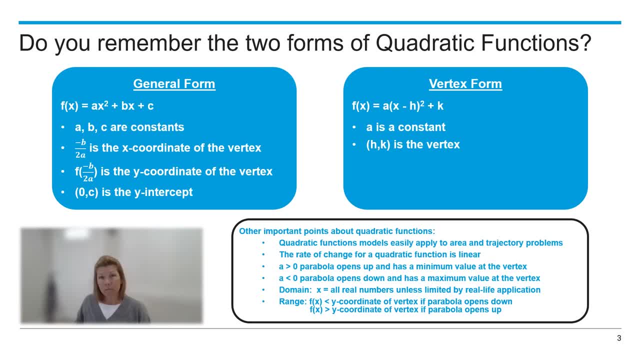 that If the? a value is greater than zero, the parabola will open up and if the a value is less than zero, the parabola will open down. Parabolas that open up have a minimum value at the vertex. 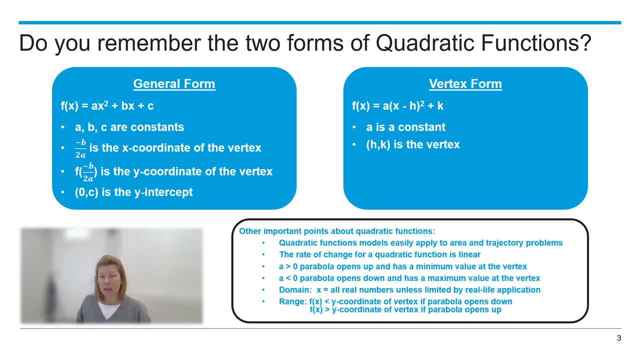 Parabolas open down. that vertex is the maximum value. it's the highest point In terms of domain. in a parabolic function or a quadratic function, the domain would be: x equals all real numbers, unless of course you're limited to a real-life application where perhaps 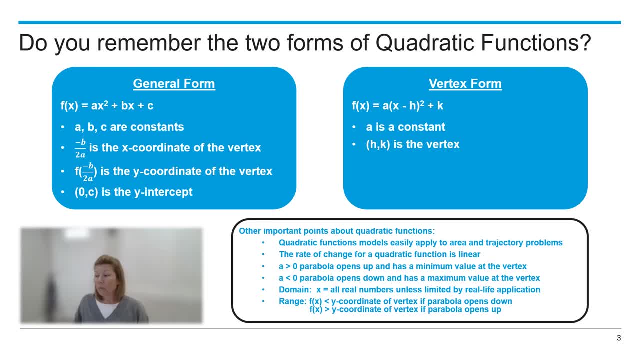 negative numbers have no meaning. The range would be: f of x is less than the y-coordinate of the vertex if the parabola opens down. or it would be: f of x is greater than the y-coordinate of the vertex if the parabola opens up. So with those gentle reminders about forms of quadratic. 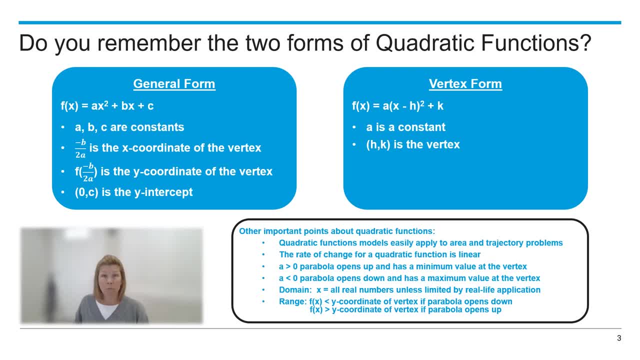 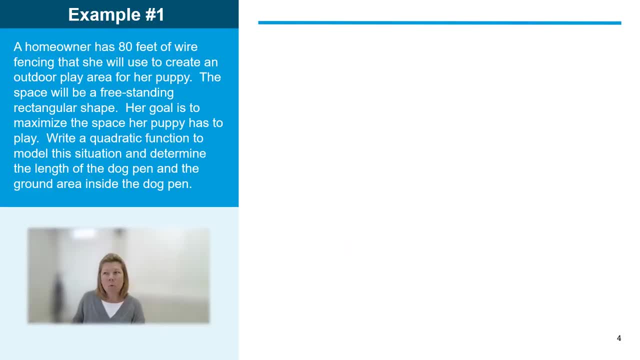 functions and graphs of quadratic functions. we'll go ahead and we'll move on to a specific example. All right, so example one: A homeowner has 80 feet of wire fencing that she will use to create an outdoor play area for her puppy. The space will be a freestanding rectangular shape. 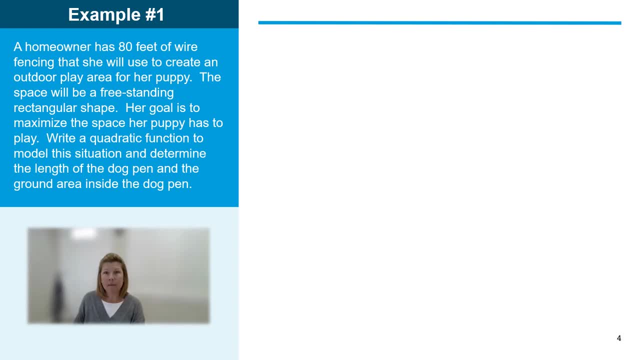 Her goal is to maximize the space her puppy will be able to use to create an outdoor play area for her puppy. Her goal is to minimize the space for her puppy's room and the space for the dog that dog will be able to use to create the room where her puppy has to play. So write a quadratic formula. 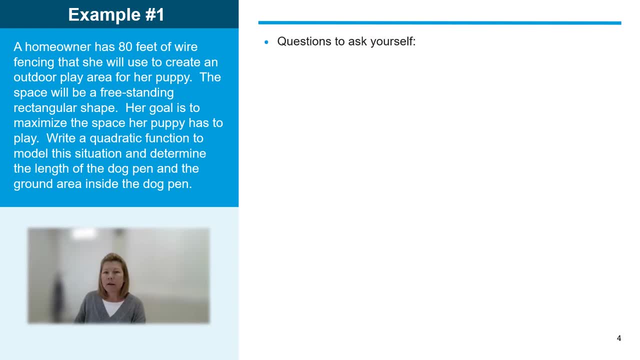 to model this situation and determine the length of the dog pen and the ground area inside the dog pen. So let's start out by asking: what questions should we ask ourselves in this particular case? And the first is: what do we know about the area of a rectangle? Well, we know that the area of a 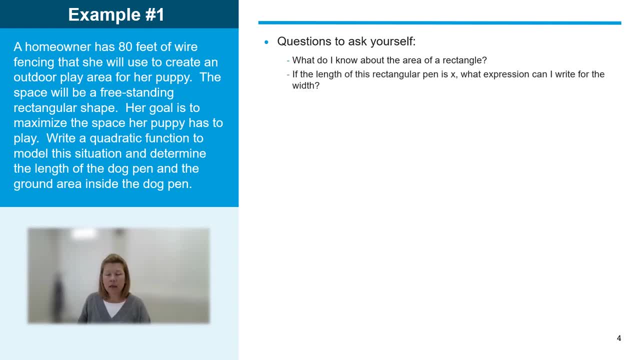 rectangle is found by multiplying length times width. The second question that we should ask ourselves to: if the length of the rectangular pen is X, what expression can I write for the length of the width and time out, because this is a common error alert. you haven't had one of those in a while, but the 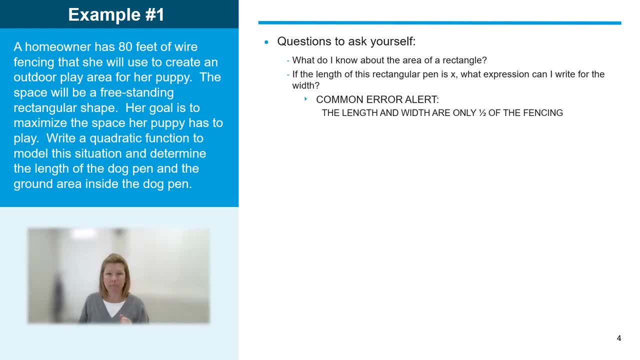 length and the width are only half of the fencing and that's because the 80 feet of fence goes around all four sides of that rectangle, but length and width account for two of the sides of that rectangle. so if the length- that means the length and width- have to add up to 40 feet of the fence, 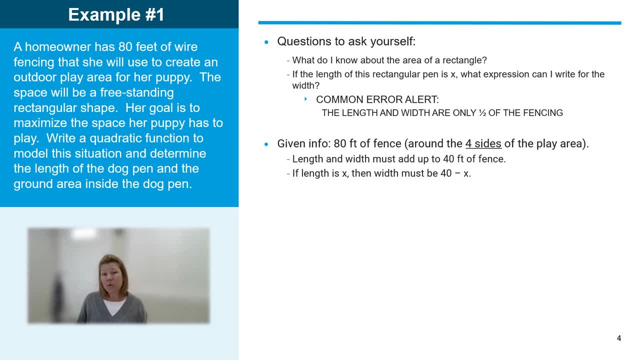 so if the length is X, then the width has to be 40 minus X, and that means that the area length times width would be X times the quantity 40 minus X. if we go ahead and distribute, that would be 40 X minus X squared. that means that we can write our quadratic function in two different. 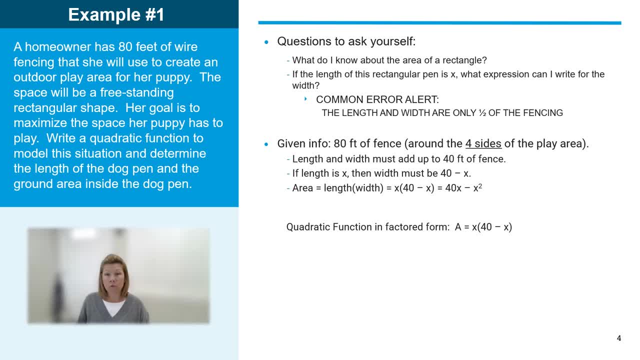 ways. we could write our quadratic function in factored form: a equals X times the quantity of 40 minus X. or we could write it in standard form: a equals negative x squared plus 40 X. the zeros of the function are at X equals 0 and X equals 40, and that means that the vertex has to be halfway in. 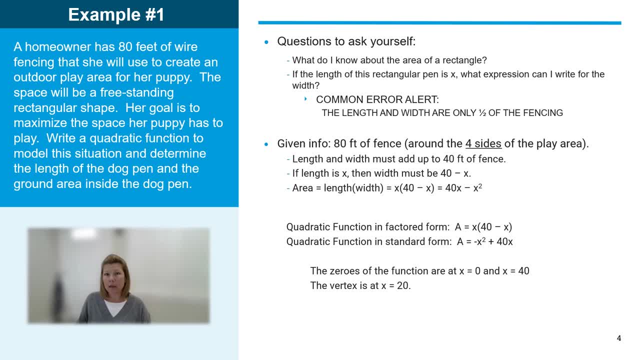 those. so the vertex has to be at x equals 20, which means that is the maximum point. if X is equal to 20, then the area would be 20 times the quantity 40 minus 20, or 20 times 20, which is 400. 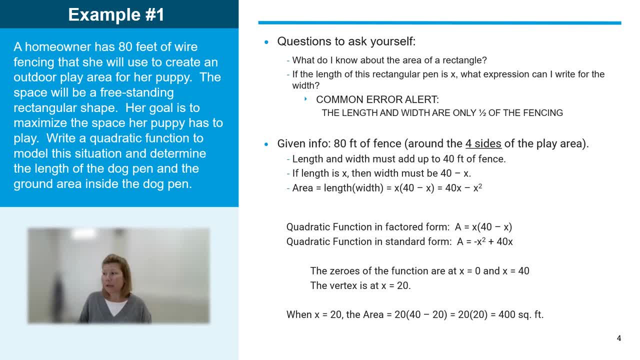 square feet. so in this particular case, the length is 20 feet, the width is 20 feet and the area of that dog pen is 400 square feet. we're adding a number there. if we do that, we can use drawing in, and then, when we middle this curve which allowed us to multiply that over puntos, this is going to be. fifteen, but then these images will be drawn. so I'm only going to highlight that little arrow in here. if you have a problem here, what you should do on this: remember the cross section and lets us write over a comma. so if you do want to write agreement, you come in and say: keep calm, don't go to the table. 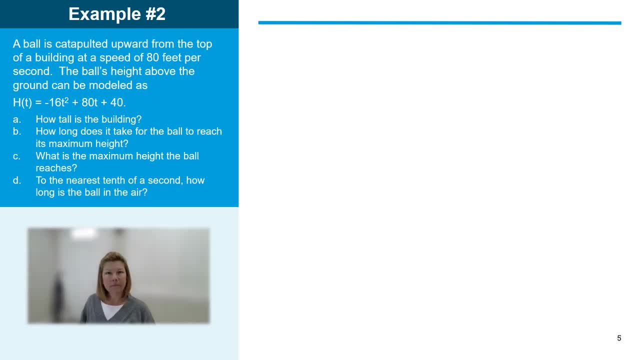 we don't want to write a number on abc company or some other naughty little age crepeudge which makes up the size of feet. Okay, and on to example two. A ball is catapulted upward from the top of a building at a speed of 80 feet per second. The ball's height above the 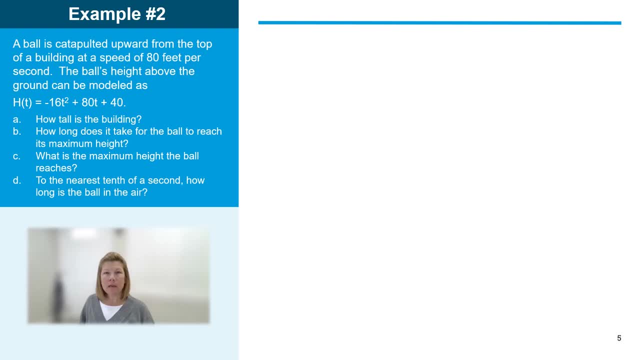 ground can be modeled as: h of t equals negative 16 t squared plus 80 t plus 40.. We're being asked to find four values: A- How tall is the building? B- How long does it take for the ball to reach its maximum height? C- What is that maximum? 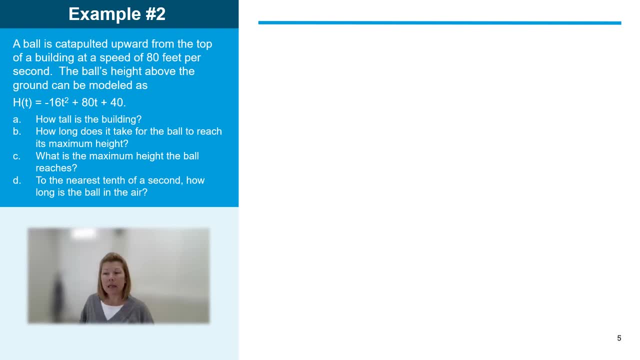 height that the ball reaches, And D To the nearest tenth of a second. How long is the ball in the air? So, as we think about this, we should be considering: what are the important points on the graph and what do they represent? Important? 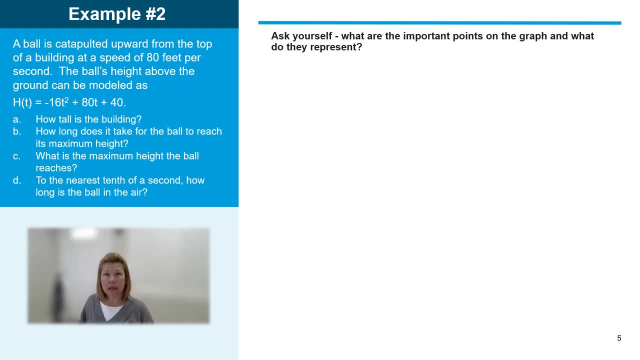 points when we graph a quadratic equation generally include things like the x-intercepts, the y-intercept and the vertex, And if you think about the fact that the vertex has a maximum height of 60 feet per second, then you should be thinking about the minimum point. So the maximum point has to do with the maximum, or? 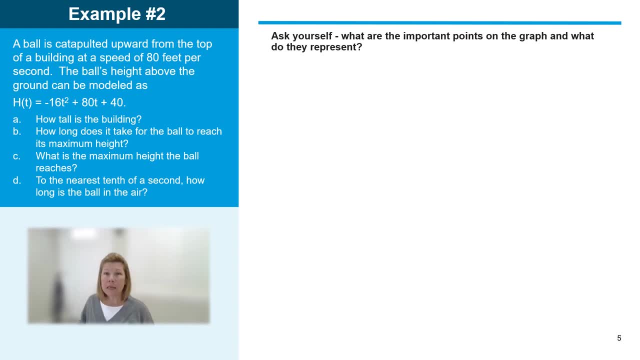 the minimum point. It's kind of a dead giveaway that B and C are both related to the vertex because they both say maximum. So A and D must have to do with the x and y-intercepts And we need to think about which is which. So when we're asked how tall is the building, 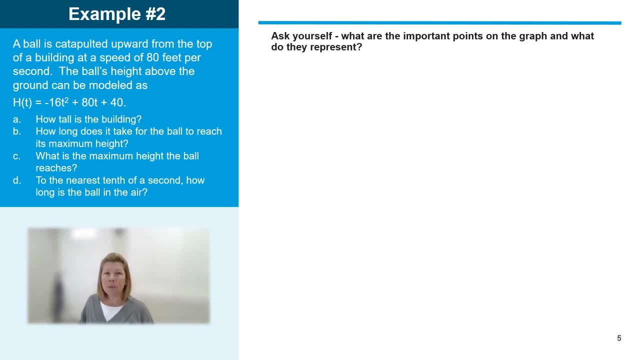 we need to ask ourselves: what do we know? We know that the ball starts on top of the building And at that point zero time has passed. So The y-intercept represents the initial height of the ball before it moves. If I put zero in place of the time, I will find out that the ball starts out at a height. 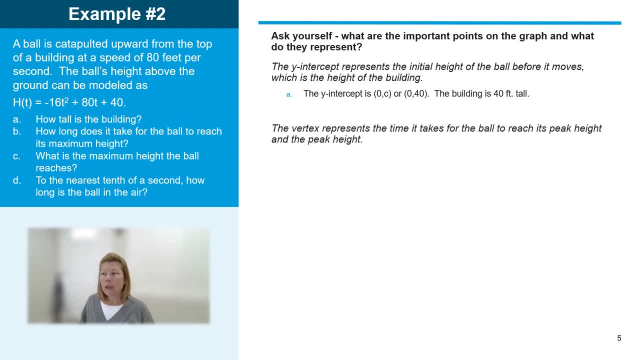 of 40 feet. As I mentioned before, the vertex represents the time that it takes for the ball to reach its peak height and what the peak height is. The x-coordinate is the amount of time, the y-coordinate is the height that it reaches. 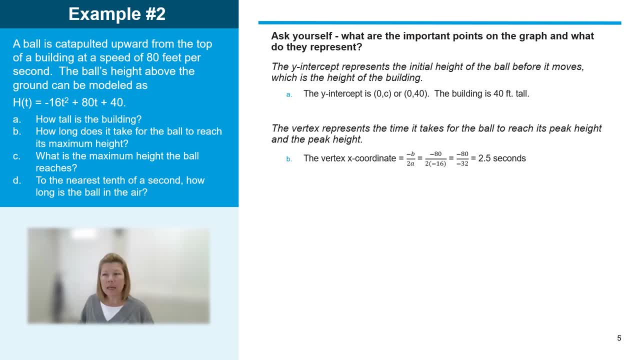 So we'll start by calculating the x-coordinate of the vertex. to answer part, The x-coordinate of the vertex is found by taking the opposite of b and dividing it by 2 times a. In this case that means negative 80 is being divided by 2 times negative 16.. 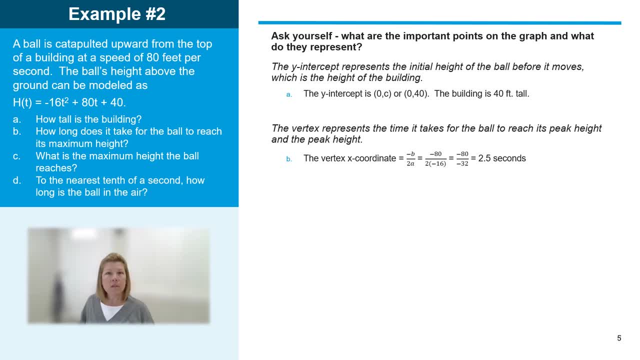 Negative 80 divided by negative 32 is 2.5, so it takes 2.5 seconds for the ball to reach its maximum height. To find that maximum height, we need to take advantage of what we know. We know that it takes 2.5 seconds, so we're going to substitute that into the equation. 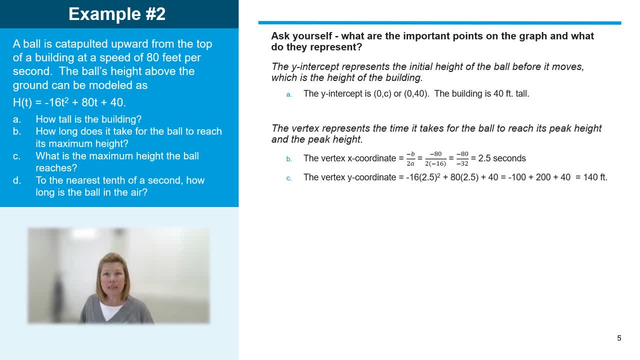 in place of the time Negative: 16 times 2.5, squared plus 80 times 2.5 plus 40, needs to be simplified using arithmetic and that will tell us that the maximum height the ball reaches is 140 feet On to part. 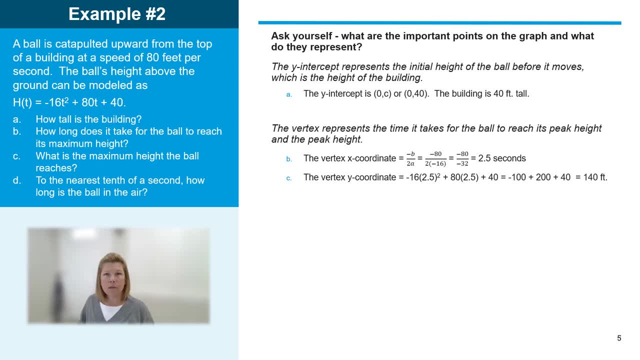 b is the ball in the air. In other words, how long does it take until the ball hits the ground or reaches a height of zero? The x-intercept is what represents the amount of time it takes for the ball to reach a height of zero or how long it's in the air. So, if we put zero, if we set, 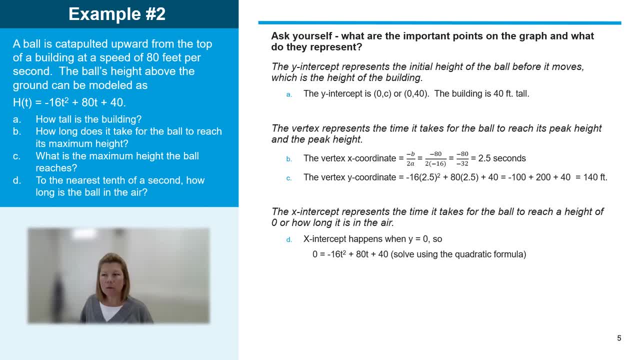 the equation equal to zero, we get: zero equals negative sixteen t squared plus eighty t plus forty. In order to solve that, we're going to need to use the quadratic formula. The quadratic formula requires us to know the values for a, b and c. In this case, a is negative, sixteen, b is. 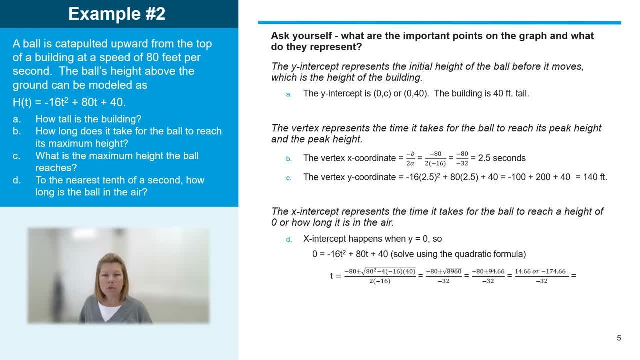 eighty and c is forty. When I substitute those values in place of the a's, b's and c's in the quadratic formula, I end up with negative eighty plus or minus the square root of 8960 divided by negative thirty-two. 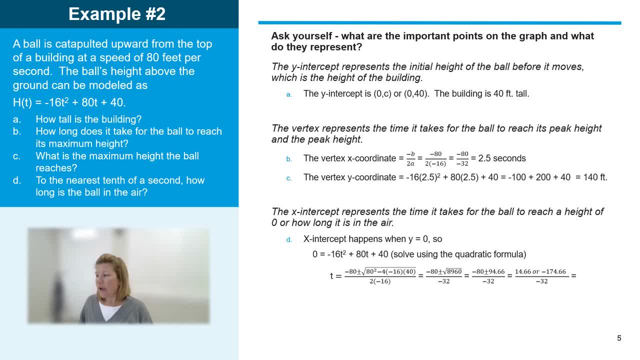 When I estimate that square root using my calculator, I get negative eighty plus or minus ninety-four point six-six. divided by negative thirty-two Adding, I get fourteen point six-six. Subtracting, I get negative one hundred seventy-four point six-six. Both of those values 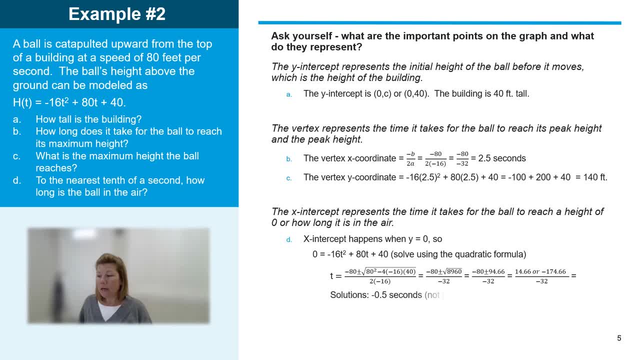 need to be divided by negative thirty-two. When I do that, I get answers of negative point five seconds, which isn't possible, And four point four seconds. So that means the ball is in the air for four point four seconds or the ball hits the ground at four point four seconds. 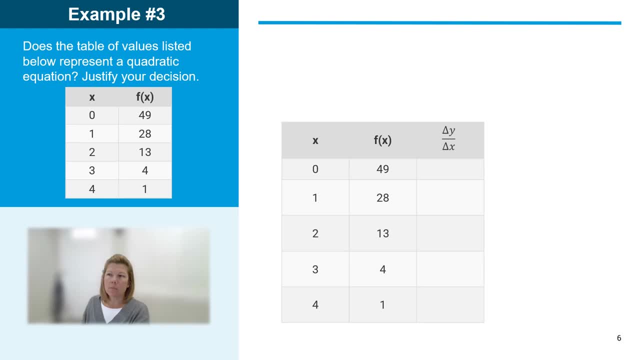 Example three: Does the table of values listed below represent a quadratic equation? justify your decision? So questions that we need to ask ourselves include: what do I know about the rate of change of a quadratic function? And, if you reflect back to the beginning of this lesson, 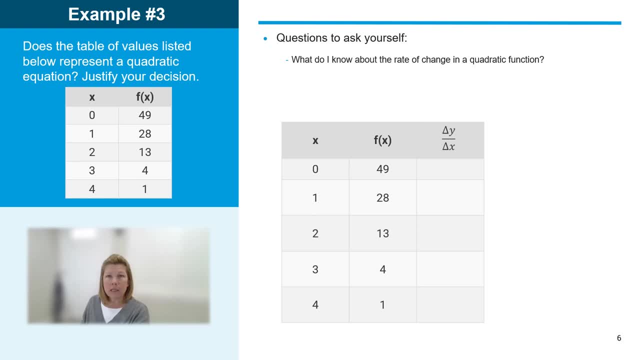 when I talked a little bit about quadratic functions, I reminded you that the rate of change in a quadratic function is linear, And so the task that we have in front of us is using this table of values to calculate the rate of change between points. 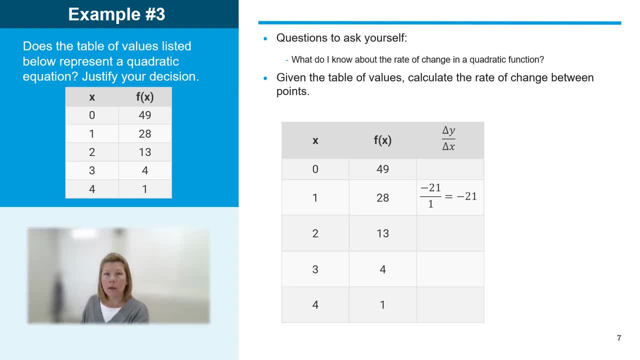 So I'm going to start with the point zero, forty-nine, and the point one, twenty-eight, and calculate the rate of change. That means I'm finding the difference in y over the difference in x. y decreases by 21,, x increases by 1, so negative 21 over 1 is negative 21.. 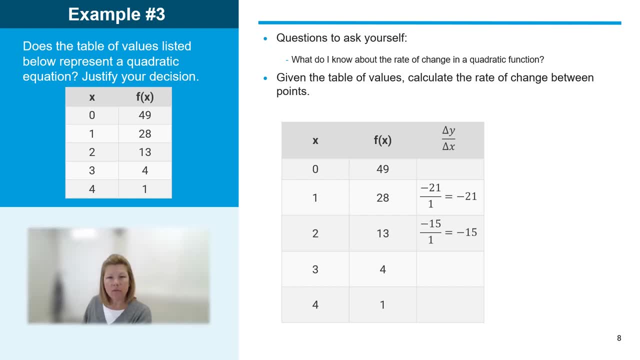 When I consider the rate of change for the next pair of points, from 128 to 213,. in this case, the change in y is a decrease of 15, and the change in x is an increase of 1.. Negative 15 over 1 is negative 15..